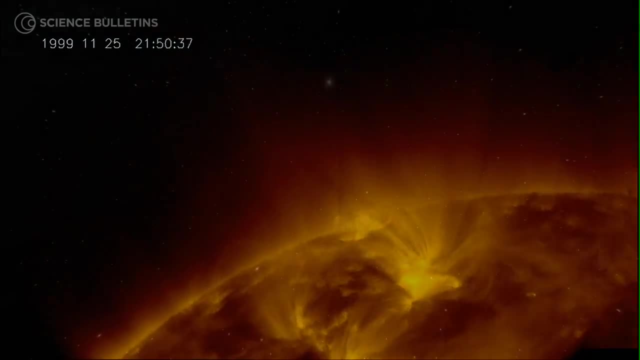 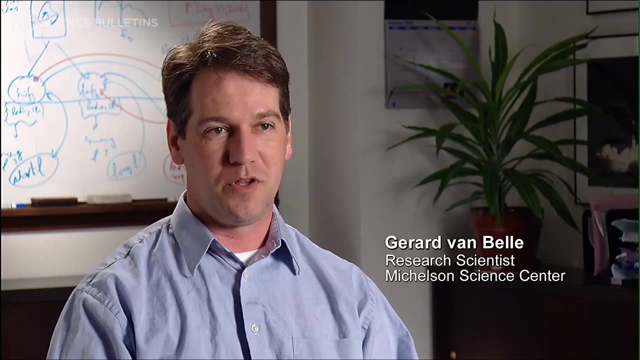 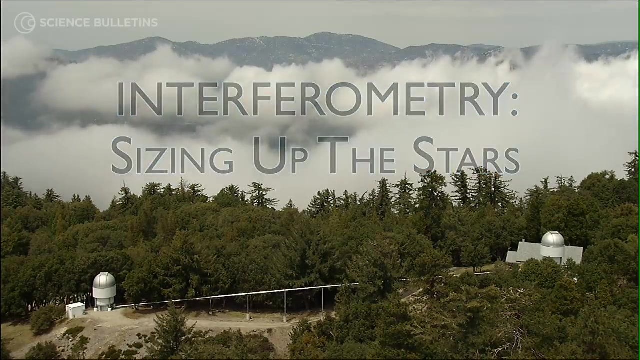 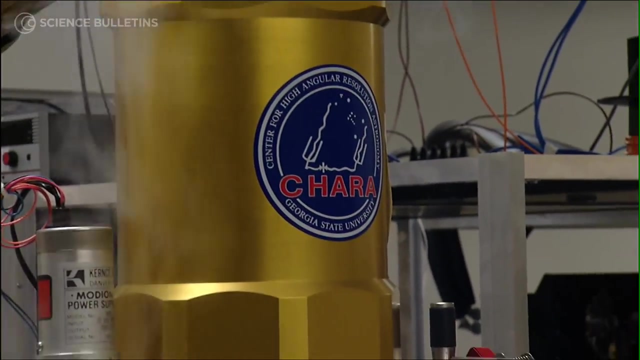 able to look at in this sort of detail, And this is where you need special techniques to look at other stars and see them in this sort of detail. that has been previously only done for the sun. CHAR stands for Center for High Angular Resolution Astronomy, which basically is the theme of 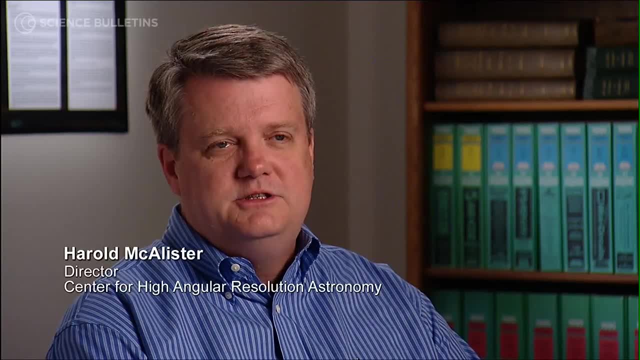 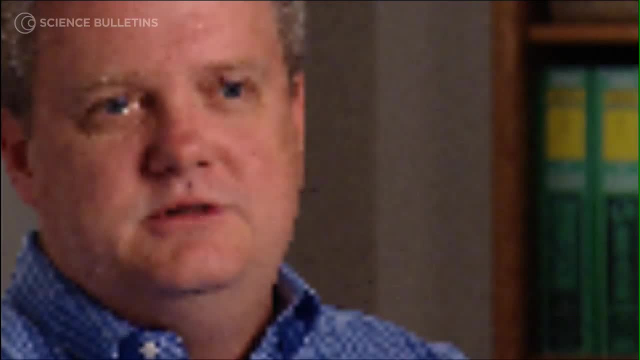 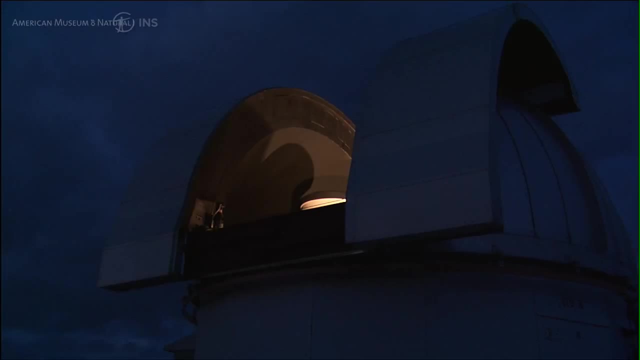 what we do. Resolution is the ability to see fine detail in distant objects, And unfortunately, distances are so great in astronomy that resolution has always been something that has been unattainable for most of the objects we look at- Stars, for example, are so far away that even with 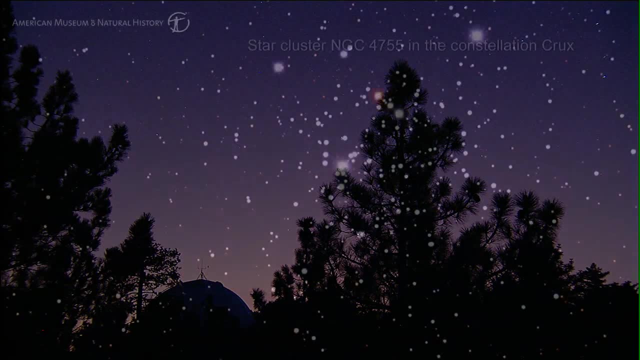 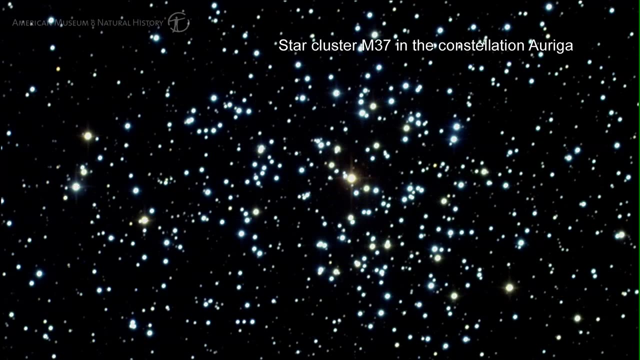 the biggest telescopes that we've ever built. most of them appear just as points of view light, But the kind of problems that we have to solve, involving measuring sizes of stars, require us to build telescopes that are not just tens of meters across. 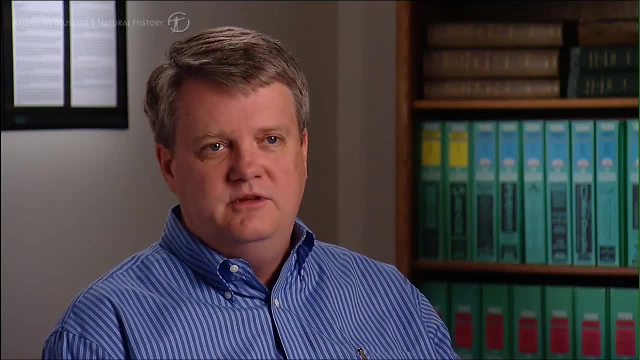 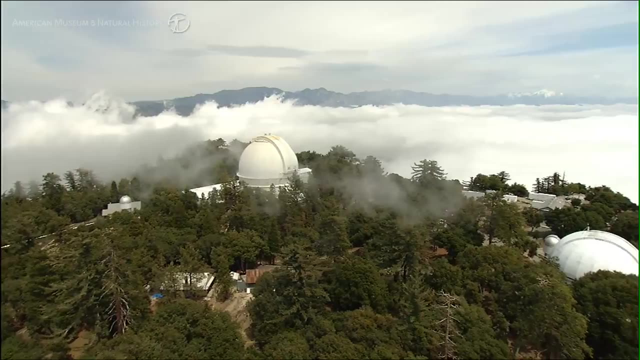 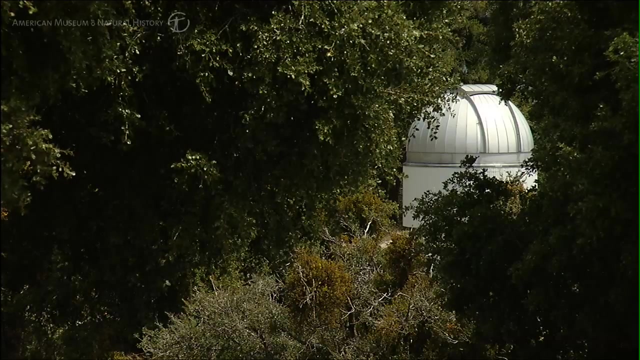 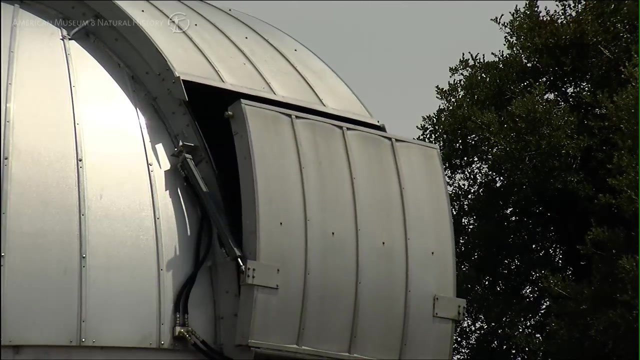 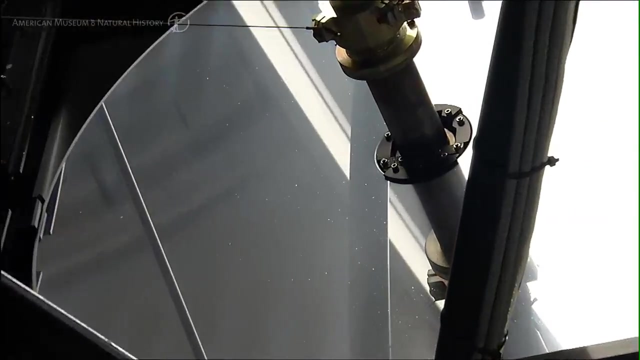 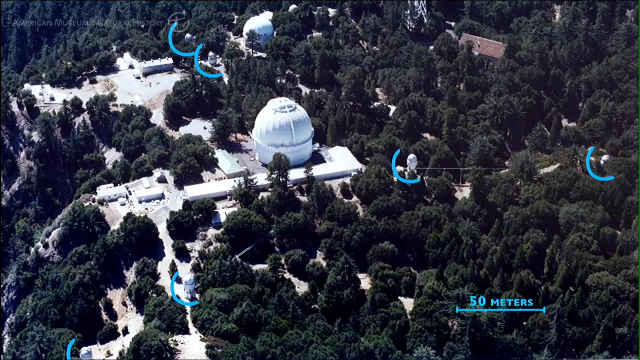 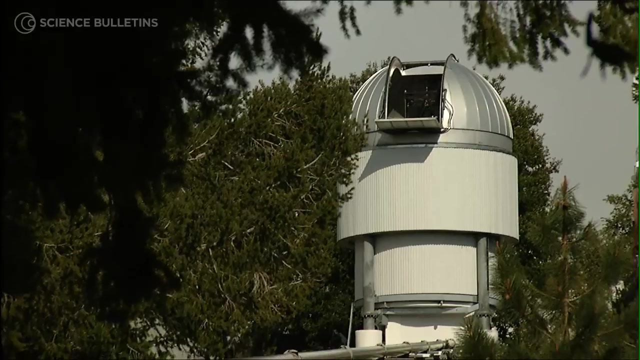 but hundreds of meters across, and those are completely unfeasible for the indefinite future. So we get around this problem by synthesizing a single giant telescope with arrays of smaller telescopes. The Char Array is a collection of six telescopes that are arranged on the ground in an area that more or less kind of covers the area that a single large telescope mirror would have, And what we then have to do is to have relay optics, many, many mirrors along the way. 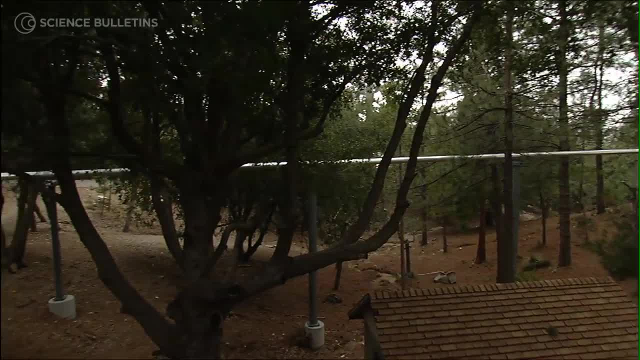 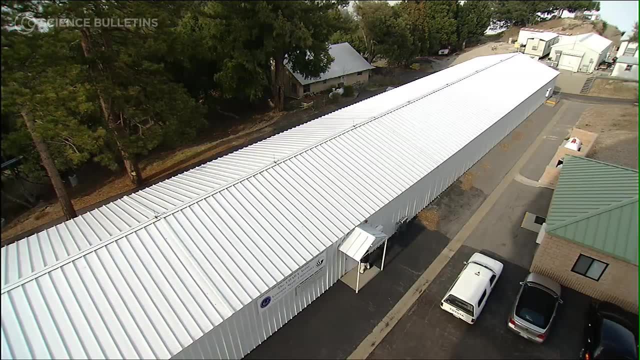 And what we then have to do is to have relay optics, many, many mirrors along the way To effectively move the beams, as if the telescopes were all placed lying on this optical mirror that we're trying to synthesize. And that's been the real. 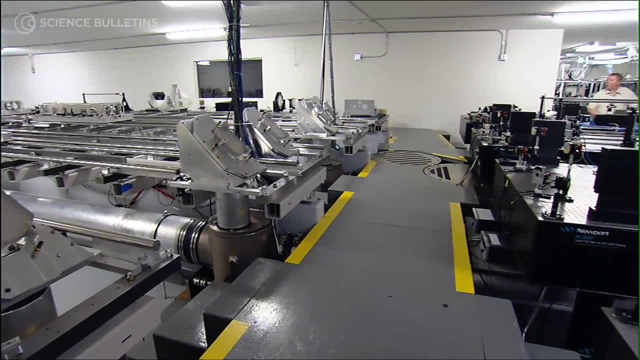 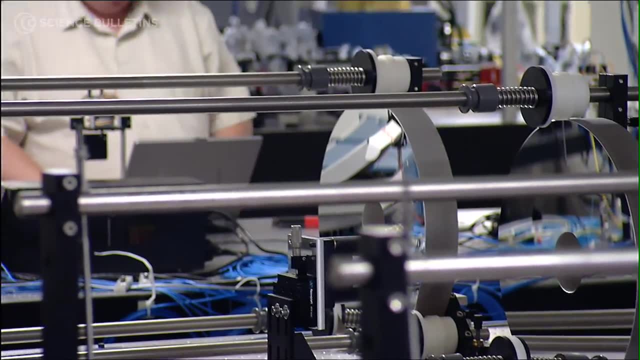 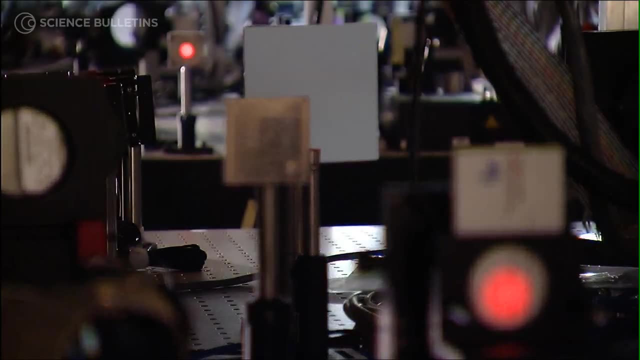 problem with interferometry being able to precisely control the beams of light to attain that synthesis of a single mirror. This is part of the daily alignment check. Essentially, we send a laser beam backwards through the system and check that it hits all the points that it. 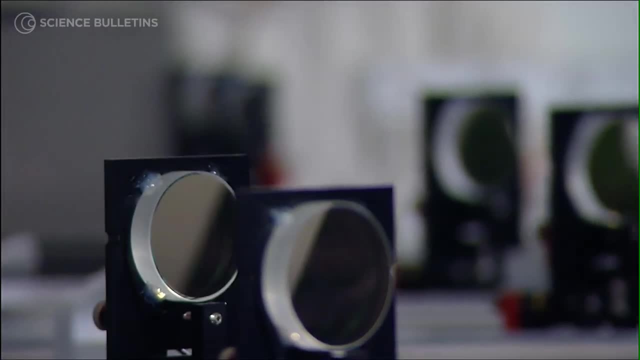 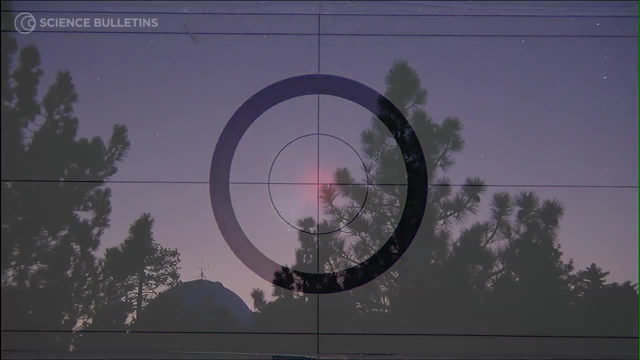 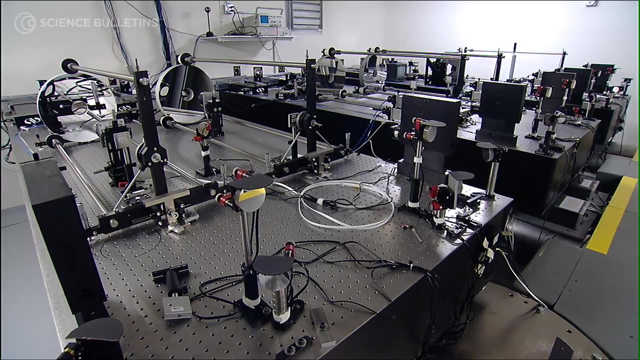 needs to hit. One of the targets is right here, spot-on. It's very important that, from the star all the way to the point inside the instrument where we bring the light beams together, that the light travel time is exactly the same Now, because the telescopes are at different elevations. 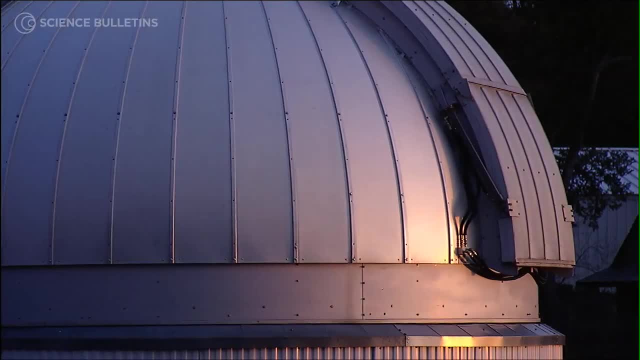 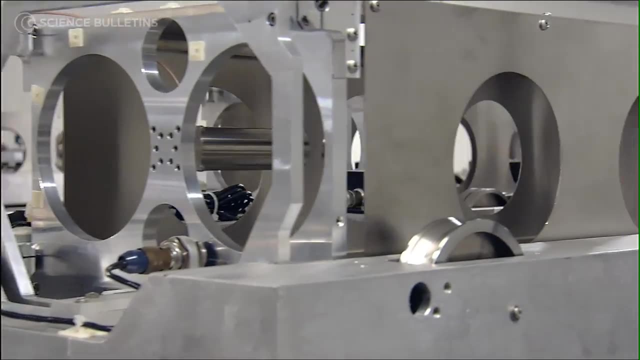 and different parts of the mountain and the earth is constantly rotating. these paths are forever changing, So we have to continuously adjust these paths within the instrument using a thing called a delay line. In interferometry, timing is everything, And that means that we have to get the light from. 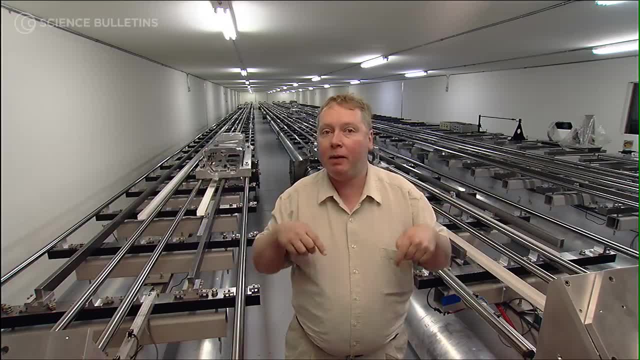 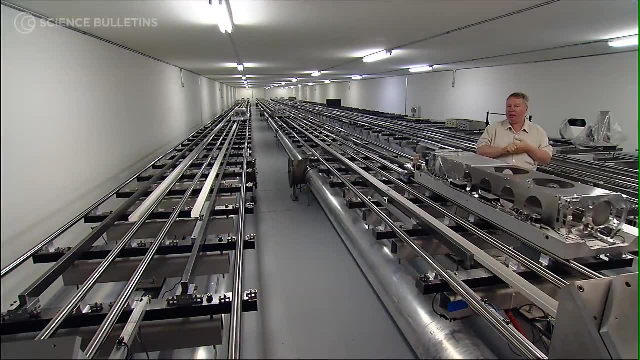 all six telescopes around the mountain into this room at the same time. While we can't control the speed of light or the time it travels, what we can do is change the path length over which it travels, And that's what this long tunnel is for. 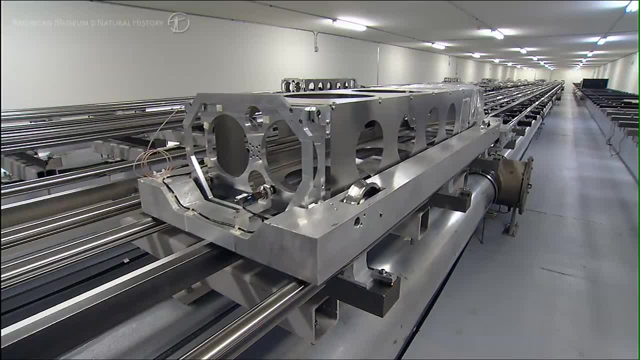 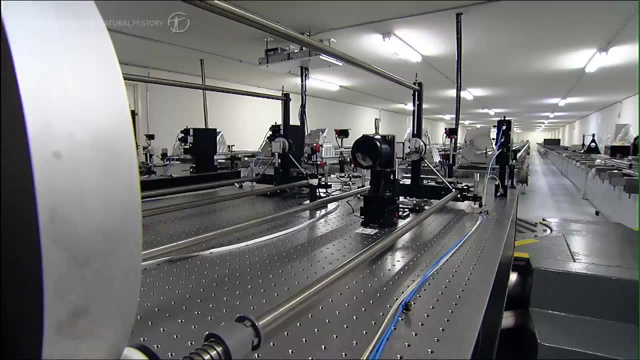 These carts are optical trombones, such that we can add and subtract path length from the telescope and make the light from each of the six telescopes arrive at the same time at the back end, so that we collect the data to make our pictures. 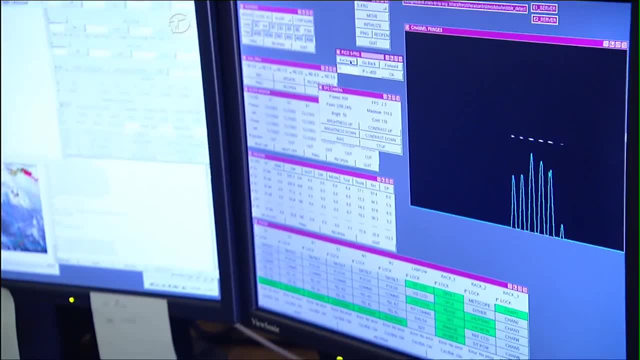 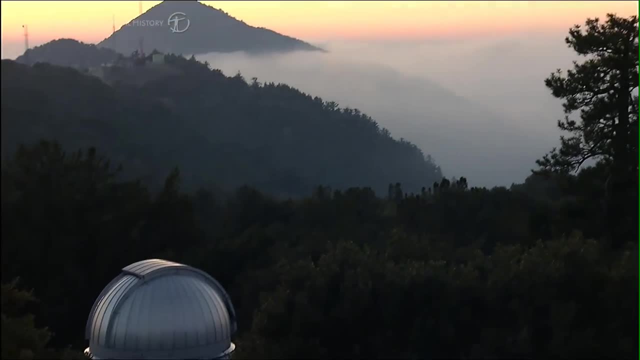 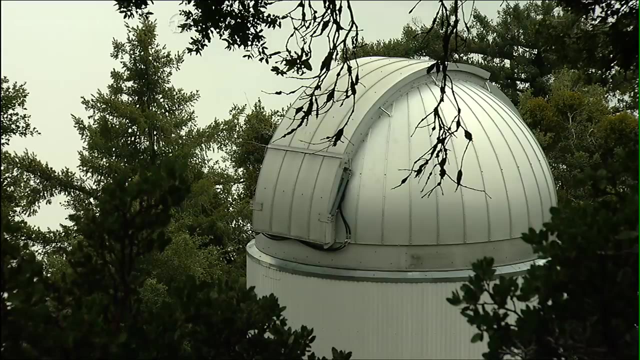 The ability to make images within interferometry is dependent upon how many telescopes you can put into the mix. As you add more and more telescopes, you get to fill in more and more pieces of this image that you're trying to synthesize as if you had a big telescope. So in the end you're never. 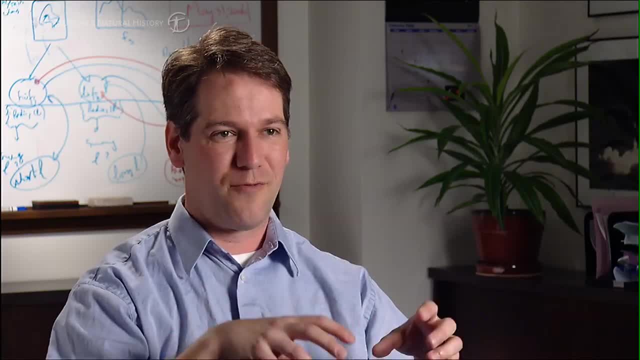 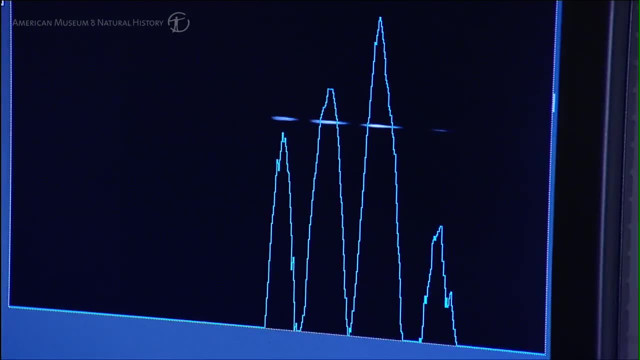 You're going to get all the way there, because you're never going to be able to put a telescope on every piece of the landscape. that is pretending to be your overall telescope, But if you do enough of it, you can actually get data that you can't get anywhere else. 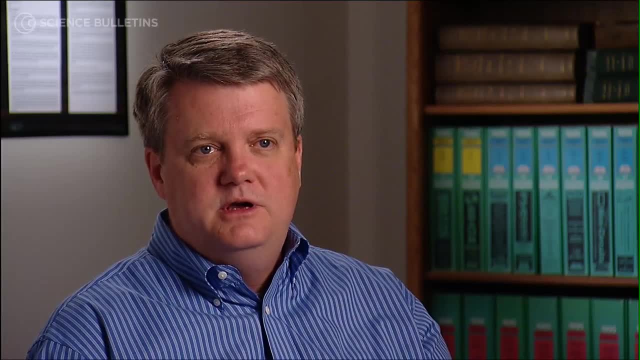 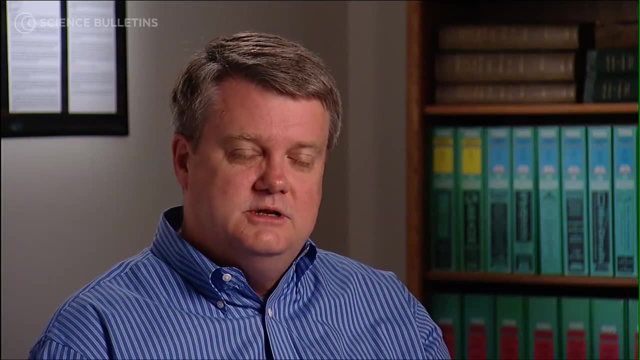 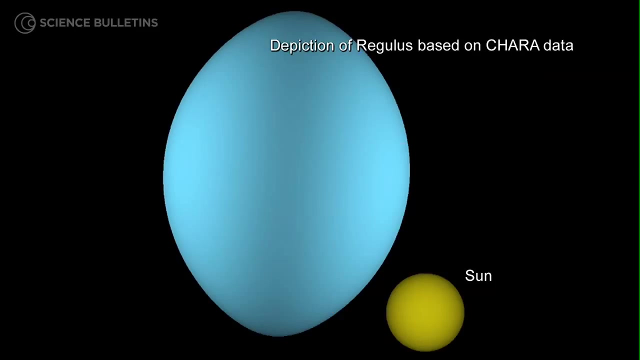 The bread and butter work, if you will, of the array is measuring these fundamental parameters for stars- their sizes, their shapes, masses, distances, luminosities and things like that- And so we produce images that are based on theoretical models that incorporate the observations. 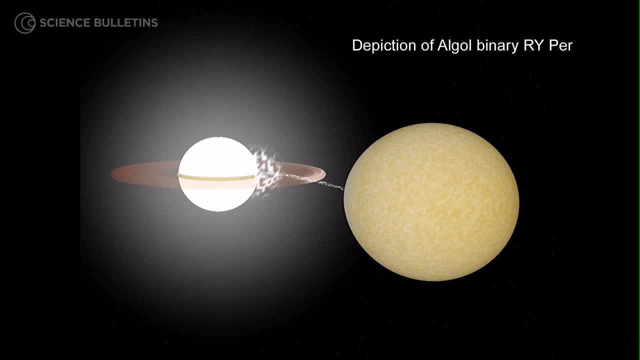 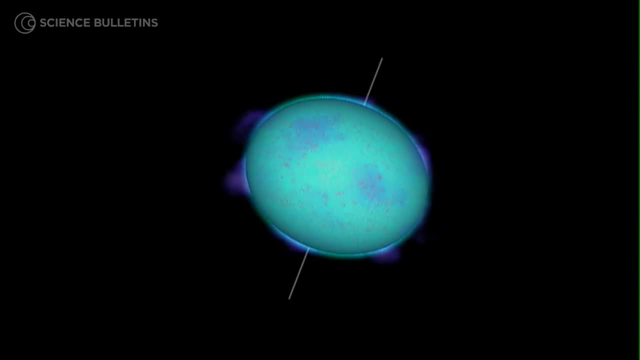 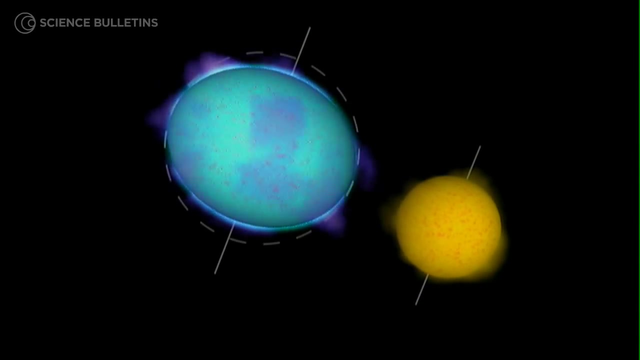 the measurements that we make. For example, we have been looking at stars that are rapidly rotating, spinning on their axes in a matter of hours rather than, in the case of the sun, about a month. And these stars are spinning so rapidly that the centripetal acceleration makes them float.